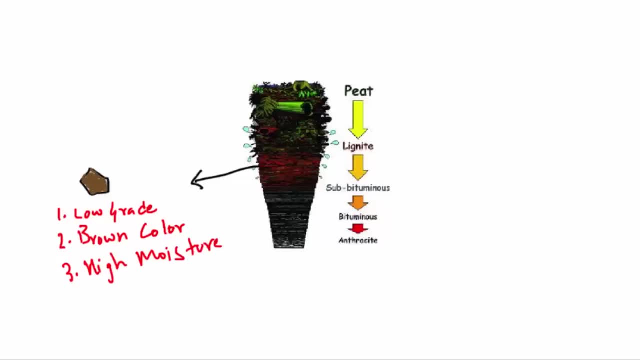 So here the decaying of plants has to take place in an area where it's wet or the water content is very high, and that place is a swampy region. It's a place that occurs along rivers or an area of low-lying land that is frequently flooded. In Hindi, we call it as: 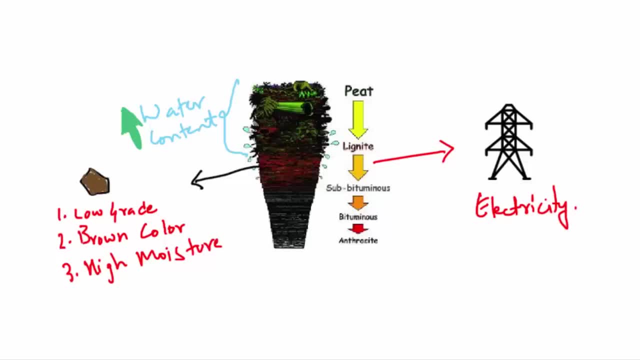 Keechar, So in this place you will find lignite coal. Now this kind of coal is found in the regions of Niveli in Tamil Nadu and they are used for generating electricity. And the second type of coal is bituminous coal. 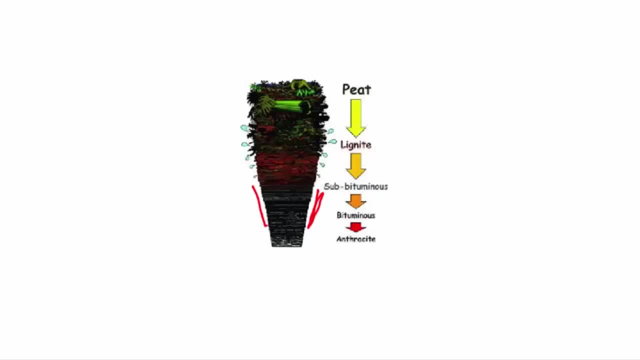 Now, these type of coal are buried deep inside the earth's crust and they are subjected to increased temperature. So we all know that as you go more inside the earth's crust, it gets hotter. the temperature increases. Therefore, it is easy to understand that this type of coal is buried deep inside the earth's crust. 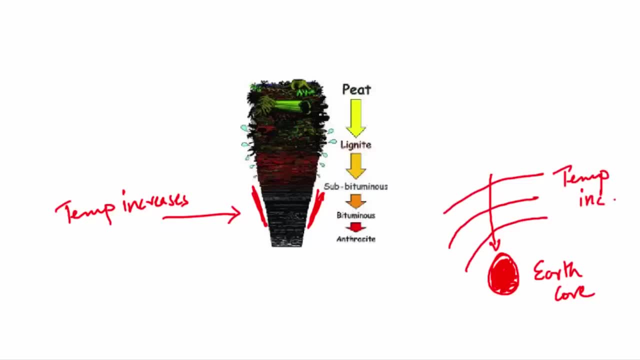 and the temperature is going to be naturally high. It is the most popular coal in commercial use, So when we say commercial, it means that it has market value. and bituminous coal is of special value because it is used for smelting of iron in blast furnaces. 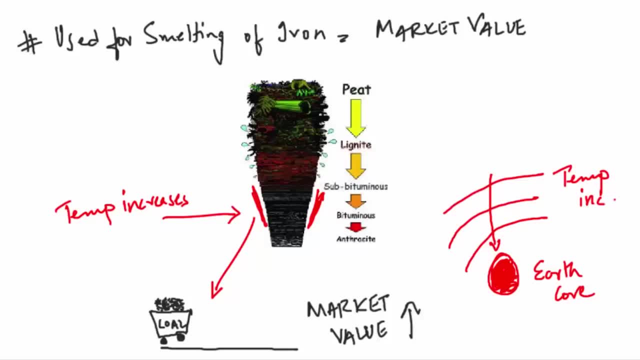 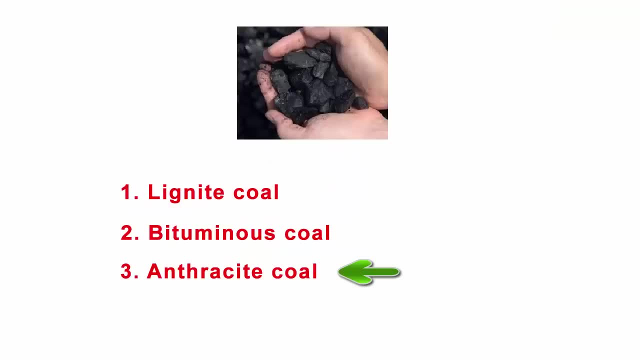 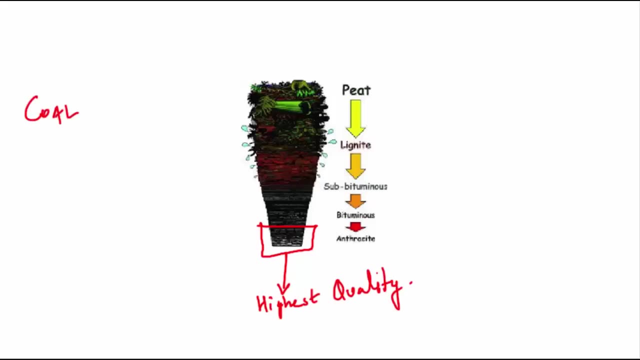 So basically, you need this kind of coal to produce iron. Hence now you understand that bituminous coal has a special value. And the third type of coal is called anthracite. Now, this is the highest quality of hard coal you can ever find. So if we were to put 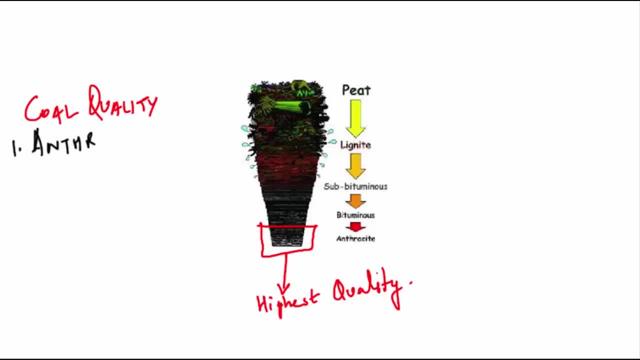 all the types of coal in order wise with respect to its quality, then the number one place goes to anthracite, because this is the highest quality of coal, And the second one will go to bituminous coal and the last one is lignite, which is low-grade brown coal. 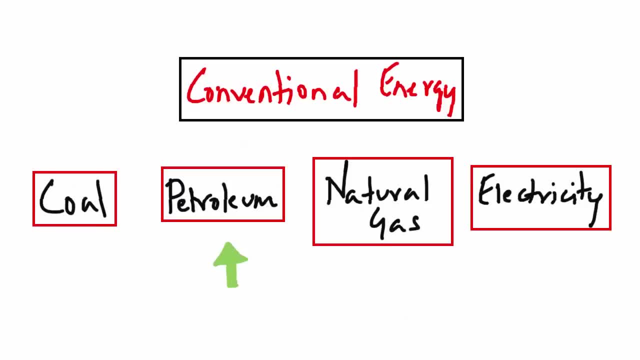 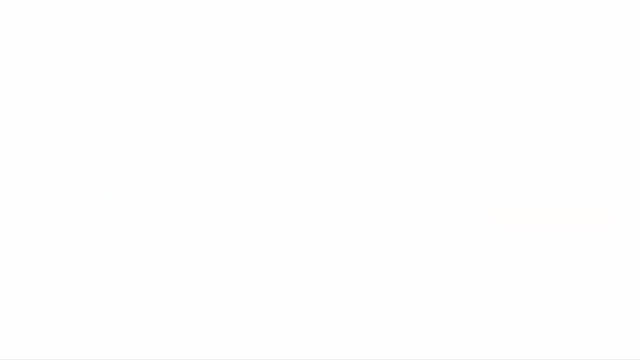 Petroleum is the second form of conventional sources of energy. Petroleum is a fossil fuel that was formed from the remains of ancient marine organisms. So what happened was algae and plants lived in shallow seas After dying and sinking to the sea floor. the organic material mixed with 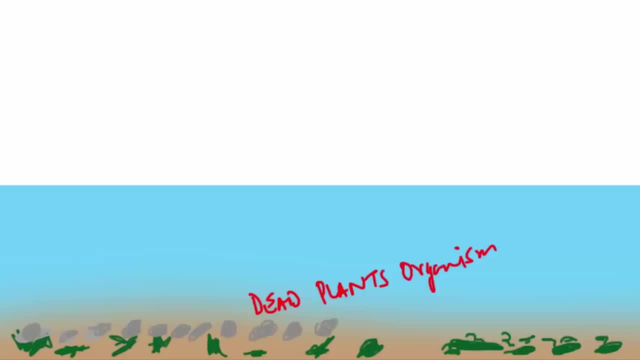 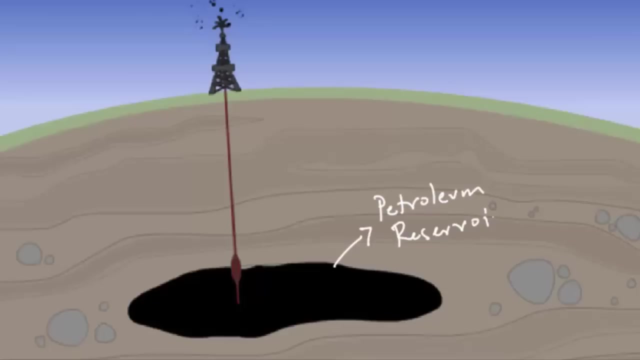 other sediments got buried and crushed under millions of tons of sediment rocks Over millions of years, under high pressure and high temperature. the remain of these organisms transformed into what we know today as fossil fuels. Petroleum reservoirs can be found beneath land or the ocean floor. Petroleum is used to make gasoline. 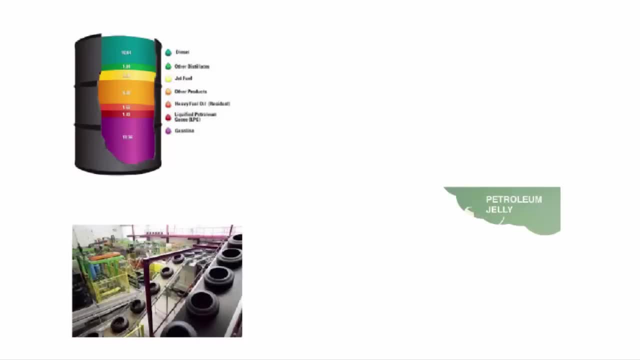 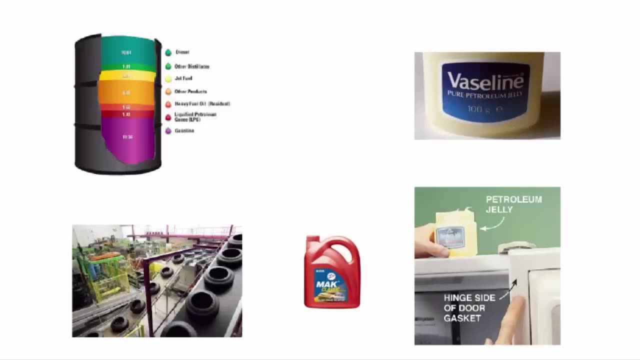 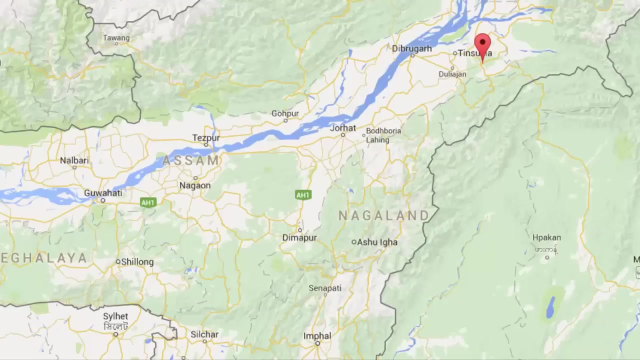 and many other important products in our everyday lives. They are used in tires, refrigerators, lubricants for machinery, moisturizing creams, etc. In India, petroleum is produced at Bombay High, Another place is Angleshwar, which is in Gujarat, And the last place is Assam. The third type of conventional 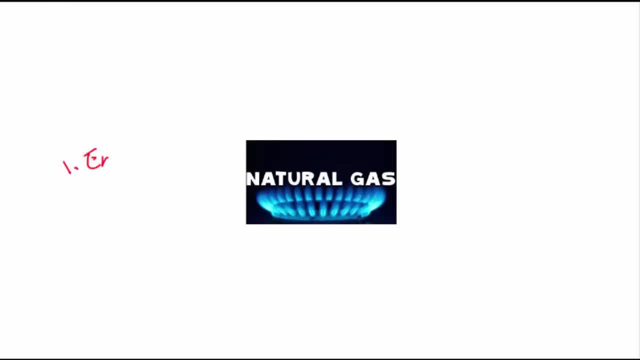 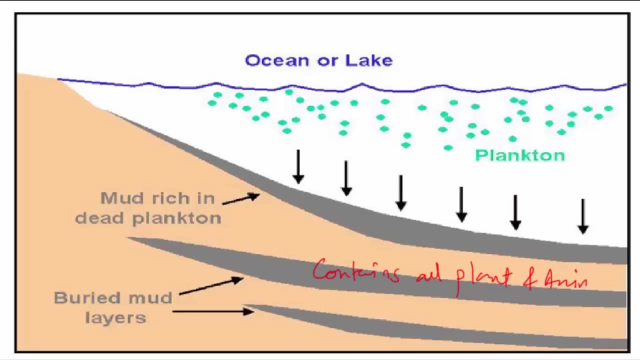 energy is natural gas. It is considered an environmental friendly fuel because of low carbon dioxide emissions, But it is associated with petroleum. In fact, its formation is also pretty much the same like petroleum, So millions of years ago, when plants and tiny sea animals were buried by sand and rock, then layers of mud. 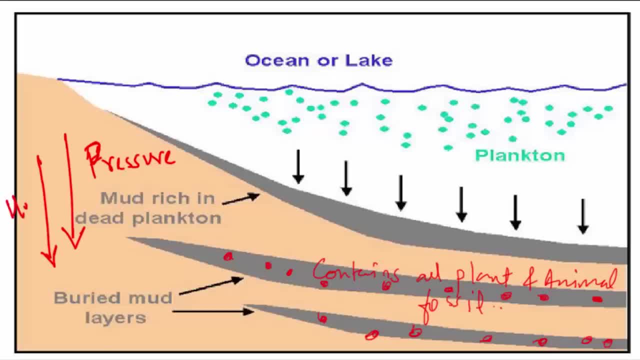 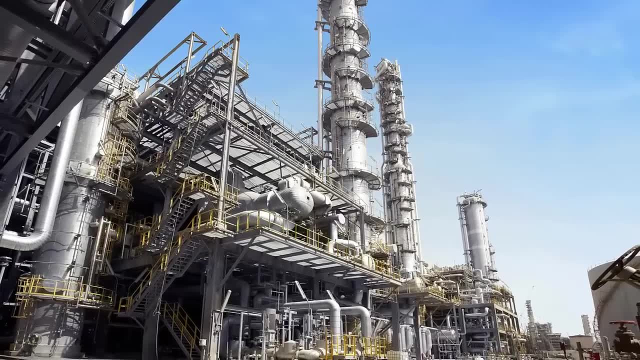 sand rock, plant and animal matter continued to build up until the pressure and heat turned them into oil and natural gas. Natural gas is used as a raw material in petrochemical industries, And petrochemical industries are those where chemicals derived from petroleum. 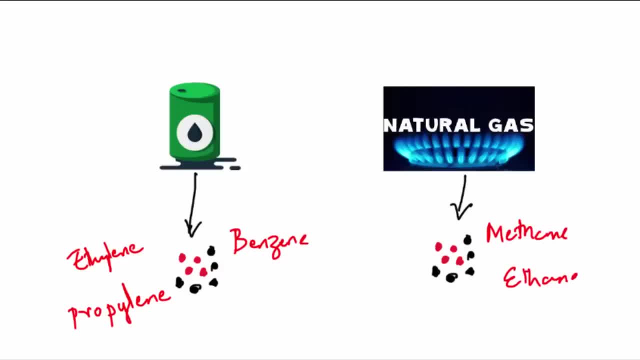 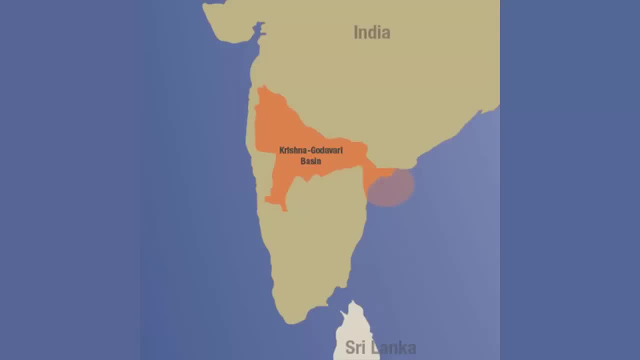 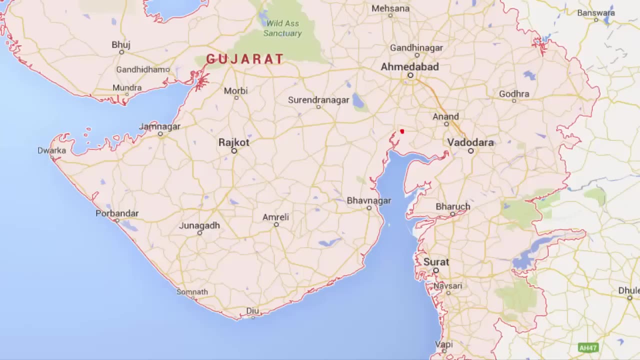 or natural gas are used in making products of fundamental human needs such as health, hygiene, housing and food. Large reserves of natural gas in India are found in Krishna, Godavari Basin, Bombay, High Andaman and Nicobar Islands and Gulf of Cambay. 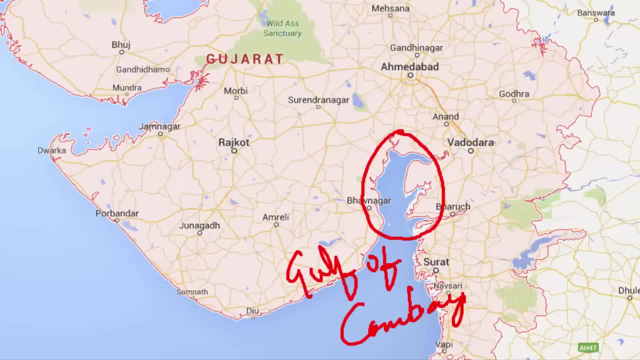 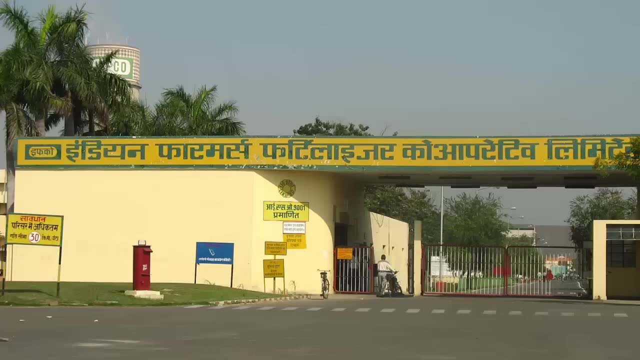 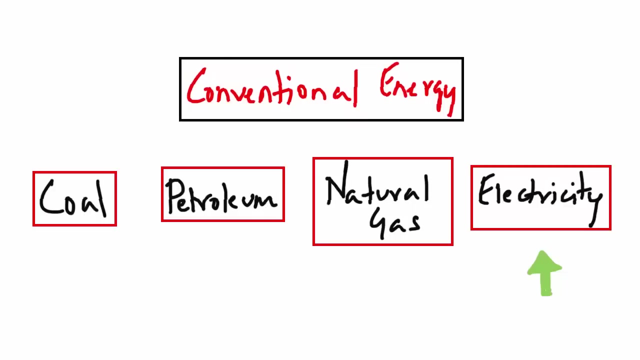 This inlet over here is referred to as Gulf of Cambay, And the other one, which is here, this, is called Gulf of Kach. Natural gas is used heavily in fertilizer industries, and compressed natural gas is used for vehicles instead of petroleum. The fourth type of conventional energy is: 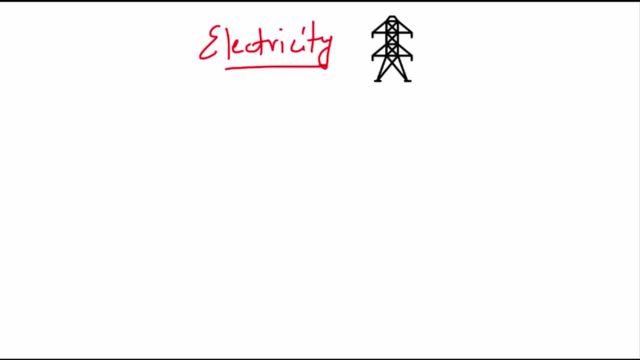 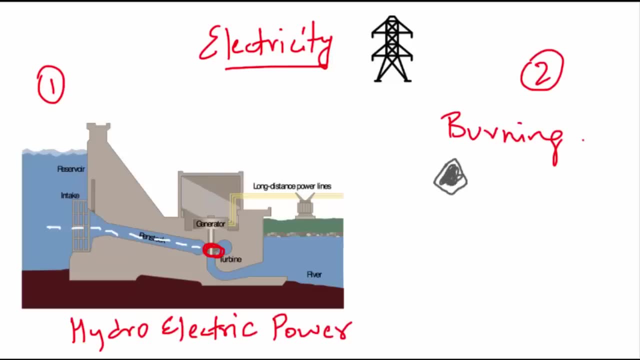 electricity. Now, electricity is generated mainly in two ways. Number one, running water, which drives hydro turbines to generate hydro electricity, And the second way is by burning other fuels such as coal, petroleum and natural gas to drive turbines to produce thermal power. So in both the manner the electricity generated is the same. 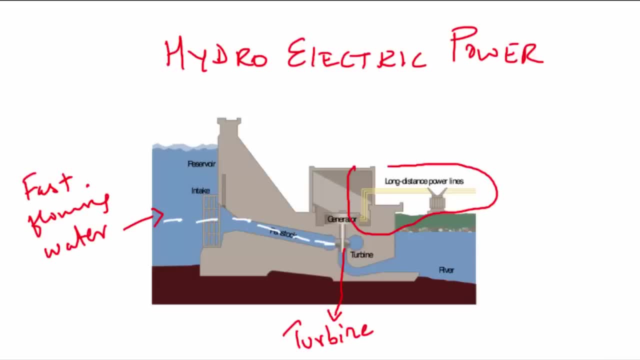 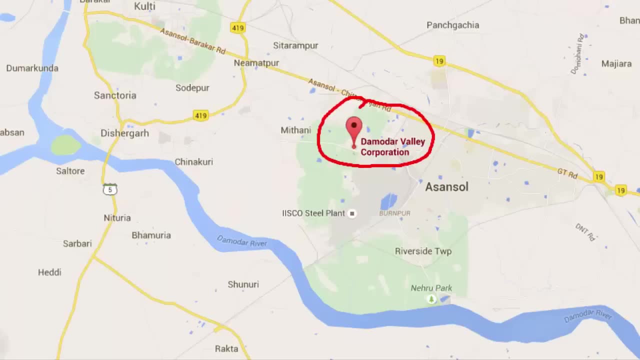 Since hydroelectricity is generated by fast flowing water. therefore it is a renewable resource, And India has a number of multi-purpose projects, like the Bhakranangal Dam, Damoda Valley Corporation, the Kopili Hydel project. These places are marked on the map. 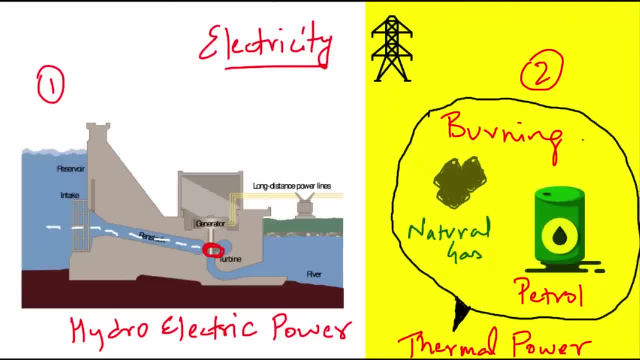 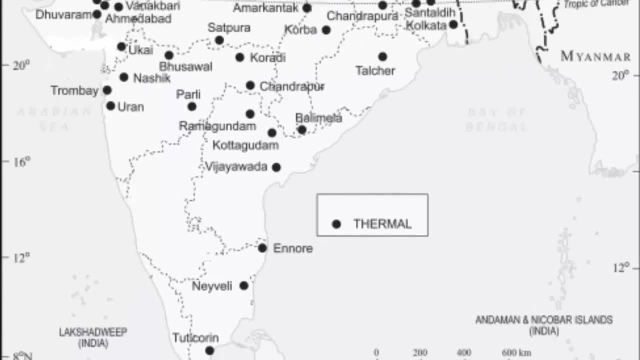 just have a look at it. And thermal electricity is generated by the water. And the second type of conventional energy is electricity is generated by using coal, petroleum and natural gas. The thermal power stations use non-renewable fossil fuels. So we have a lot of thermal power plants in India. 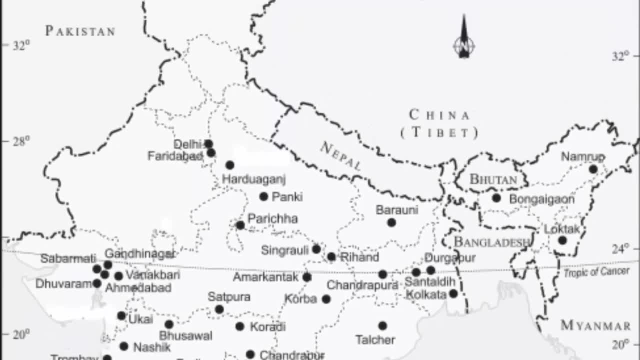 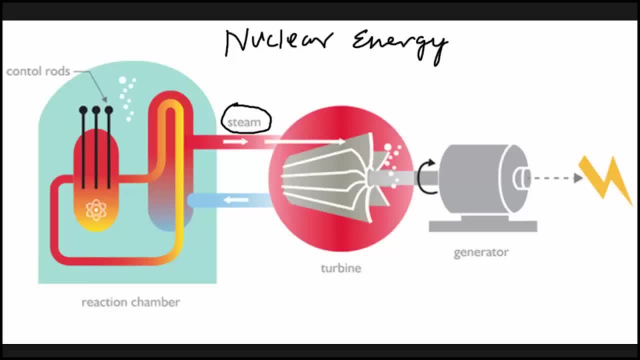 Have a look at this map and you should see some of the places. And the last form of conventional energy is nuclear or atomic energy. So in a nuclear-fueled power plant, water is turned into steam, which in turn drives turbine generators to produce electricity. The difference is the source of heat. 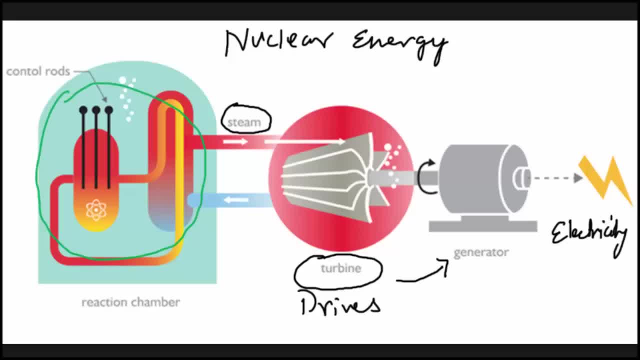 In nuclear power plants there is a lot of heat generated by the water. So in a nuclear powered power plant, water is turned into steam, which in turn drives turbine generators to produce electricity. The difference is the source of heat. the heat to make the steam is created when uranium atom splits, which is also called fission. 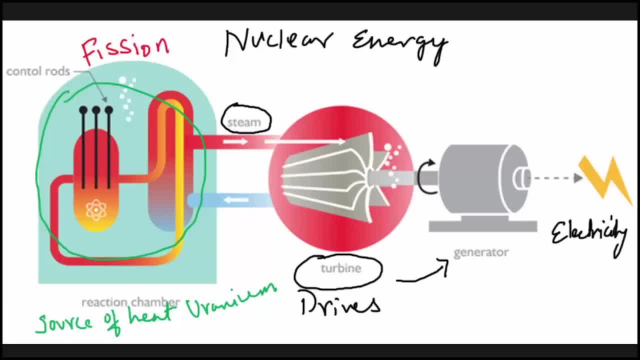 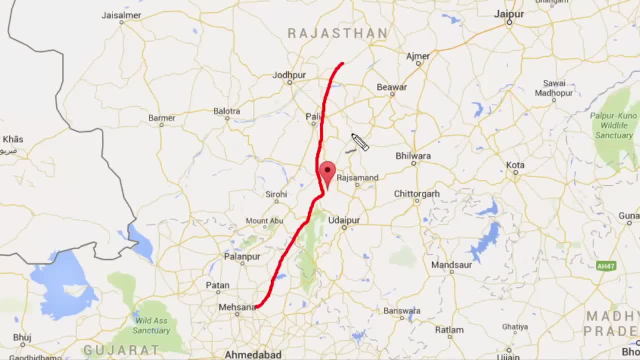 So in nuclear fission, energy is released in the form of heat, and this is used to generate electric power. Uranium and thorium, which are available in Jharkhand and the Arawali ranges of Rajasthan, are used for generating atomic or nuclear power. 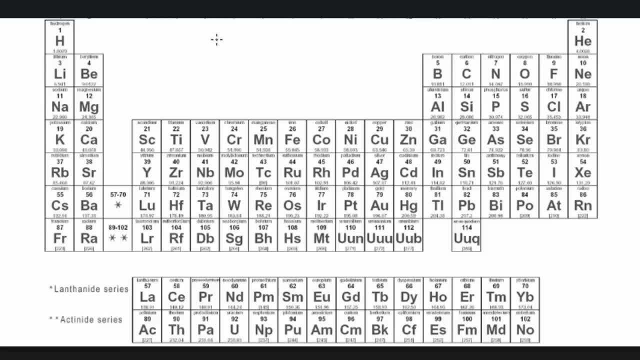 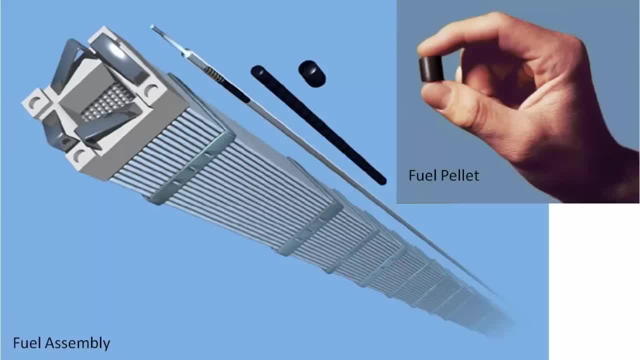 The monazite sands of Kerala is also rich in thorium. So thorium is a chemical element which is highly radioactive and it is also a primary fuel for many of the nuclear reactors. So some of the nuclear power plants in India are: just have a look at this map and you should see some of them. 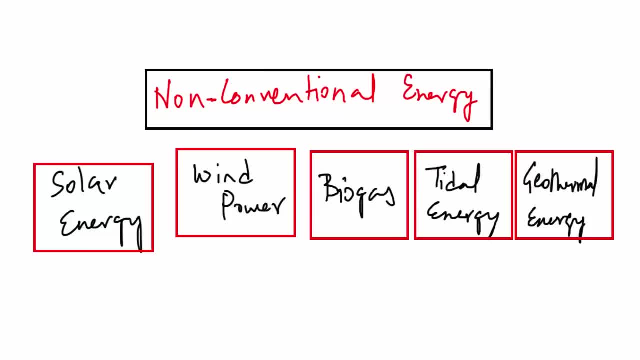 Now let's read about the second part of this video: non-conventional sources of energy. The energy generated by using wind, tides, solar, geothermal, heat and biomass is referred to as non-conventional energy. These energy sources are renewable and ecologically safe. 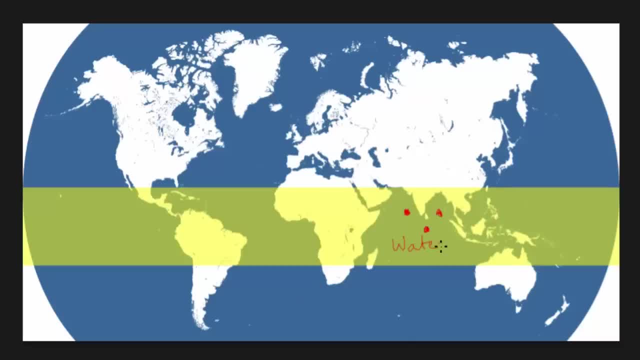 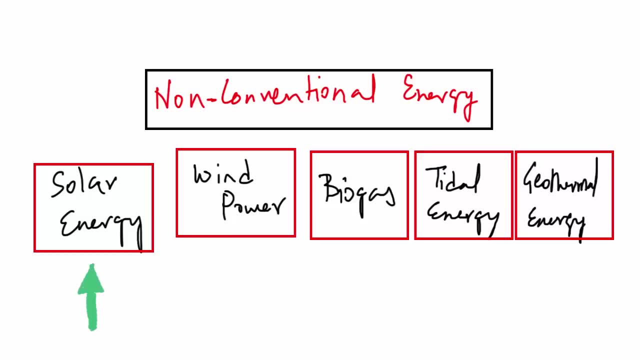 India is blessed with an abundance of solar. It is also known as solar energy. It is also known as solar energy because solar energy is used to generate energy from sunlight, water, wind and biomass. Now let's read about some of the non-conventional sources of energy. 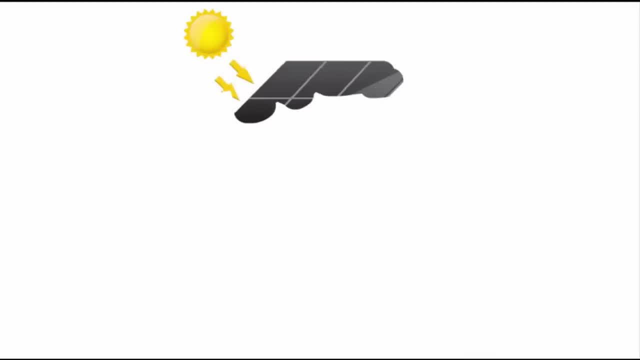 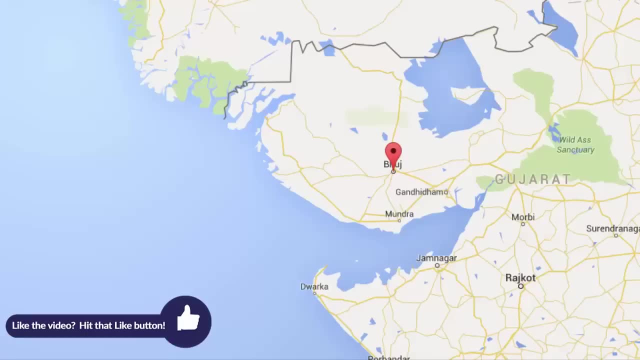 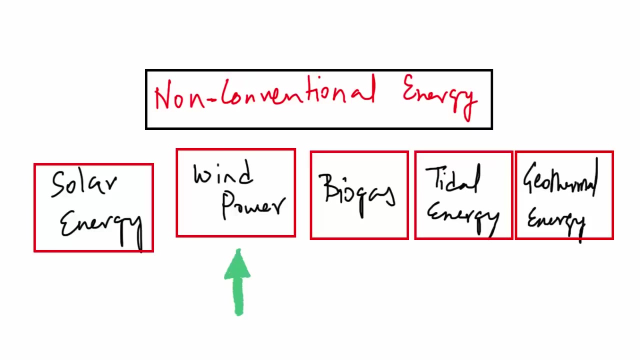 The first one is solar energy. Photovoltaic technology converts sunlight directly into electricity. Photovoltaic is also referred to as solar cells. They convert the energy of light directly into electricity. The largest solar plant of India is located at Madhapur, near Bhuj, Gujarat. 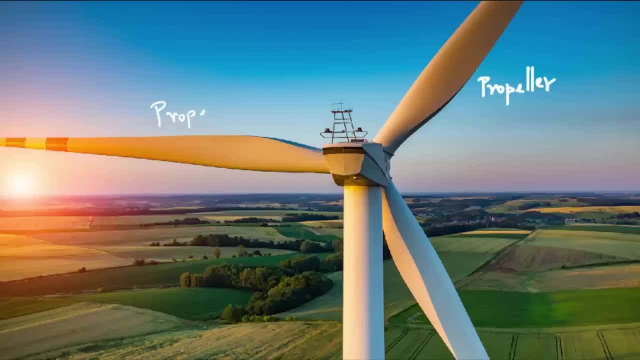 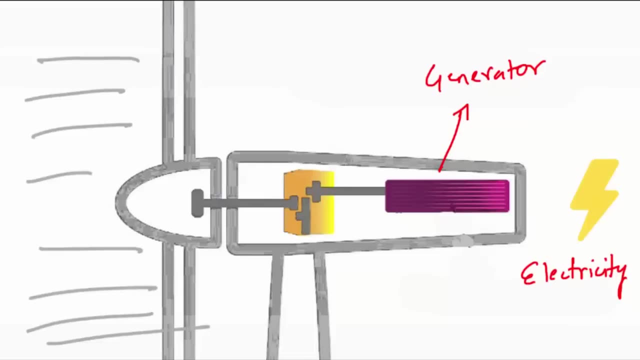 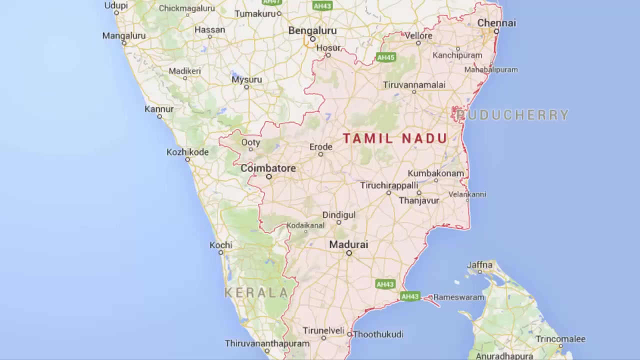 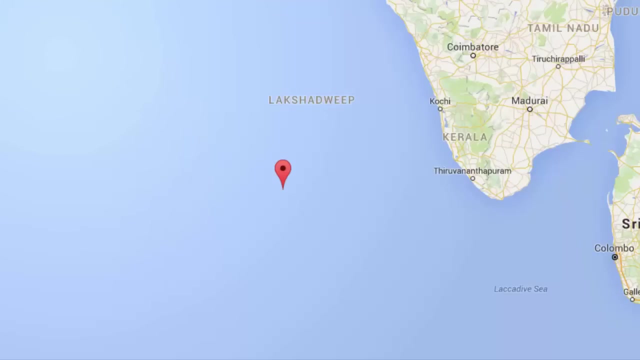 This is done by using a large wind turbine, usually consisting of propellers. The turbine is connected to a generator to generate electricity. As the wind passes the turbines, it moves the blades, which spins the shaft, and that generates electricity. The largest wind farm cluster is located in Tamil Nadu, Andhra Pradesh, Karnataka, Gujarat, Kerala, Maharashtra and Lakshadweep. 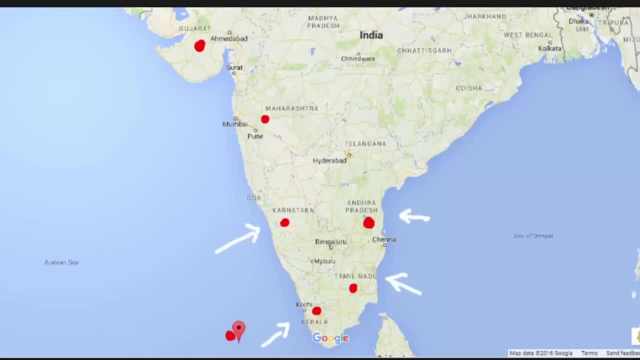 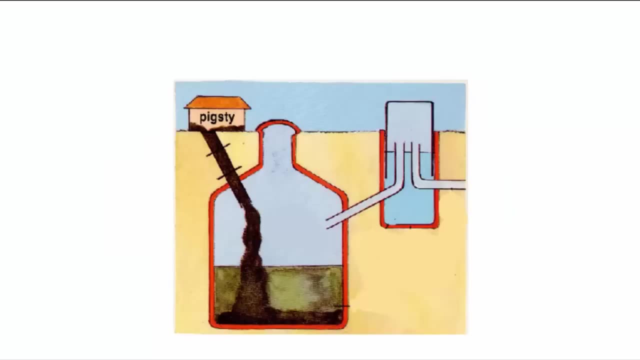 And if you look at these places, they all are located at coastal region, Hence wind from sea is in abundance. The third non-conventional energy source is biogas. Biogas is produced in a biogas plant. Shrubs, farm waste, animal and human waste are dumped into the biogas plant. 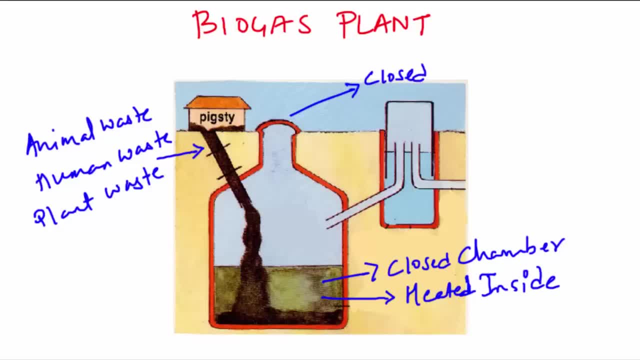 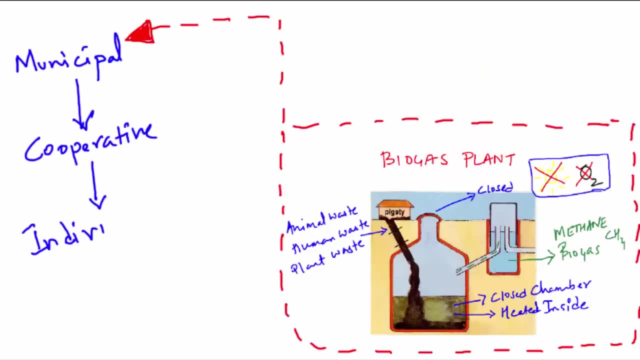 It is then heated to a certain temperature. The leftover is decomposed by the microorganisms under exclusion of light and oxygen. The final product is biogas, and its main element is methane gas. Biogas plants are set up at sea. Biogas plants are set up at municipal, cooperative and individual levels. 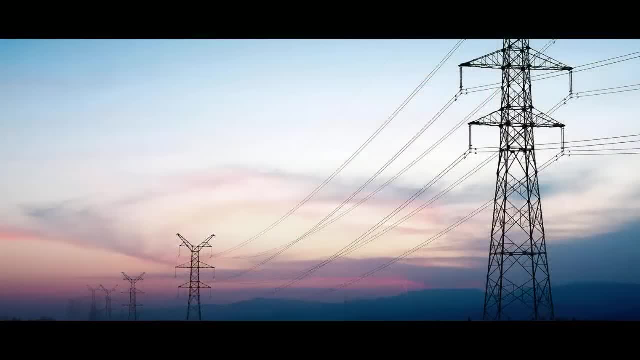 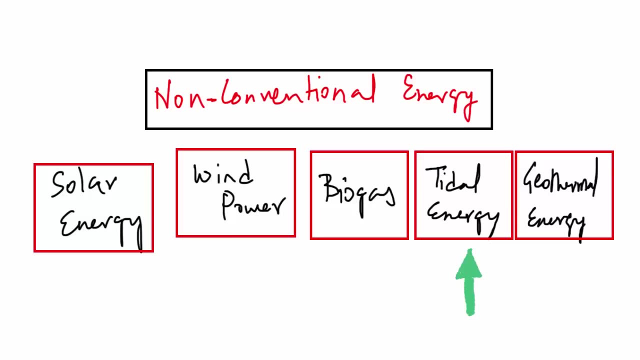 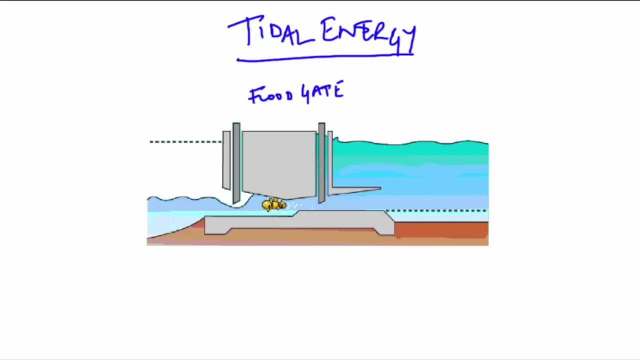 It is very beneficial for rural farmers because it not only produces energy, but it also produces fine quality manure. The fourth non-conventional energy source is tidal energy. Floodgate dams are built across inlets. During high tide, water flows into the inlet and gets trapped when the gate is closed. 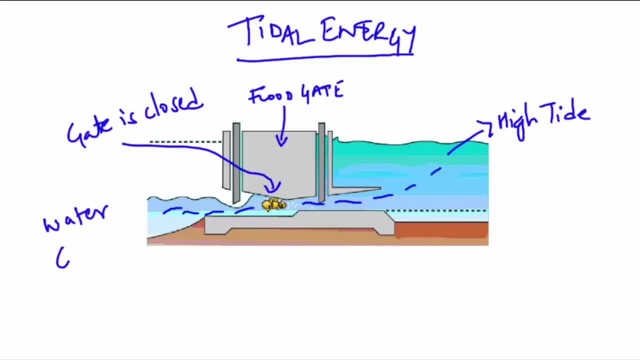 After the tide falls outside the floodgate, the water retained by the floodgate flows back to the sea via a pipe that carries it through a power generating turbine. If you see, it's purely using natural force, along with the help of mechanical process, to generate electricity. 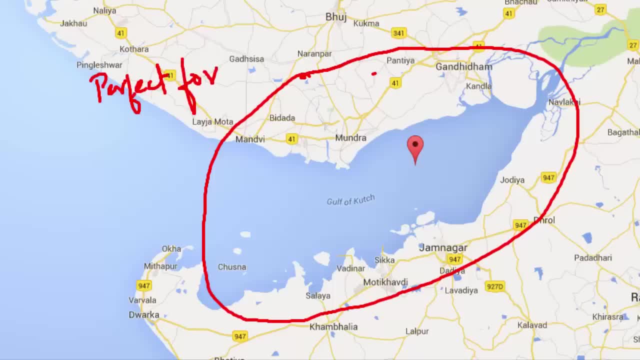 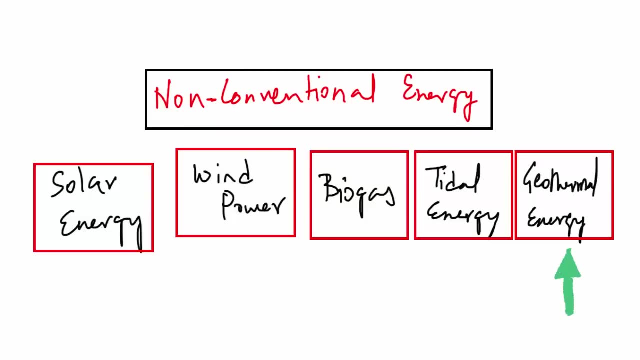 In India, the Gulf of Kutch provides ideal conditions for utilizing tidal energy. Last but not the least, geothermal energy is another form of non-conventional energy source. When we break the word geothermal, we get geo, that is referred to as earth.